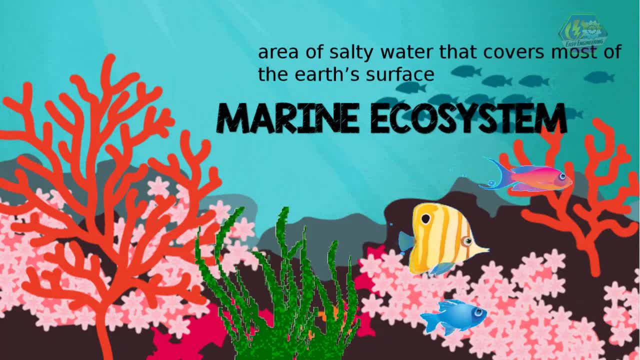 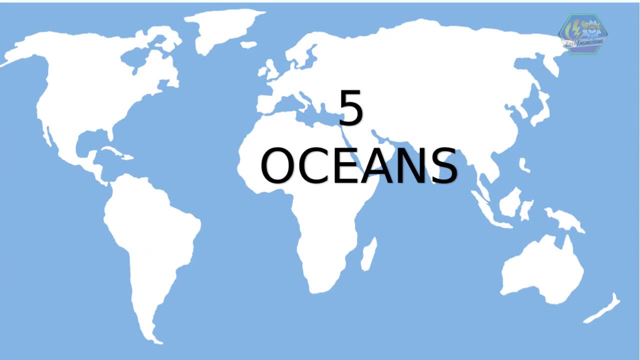 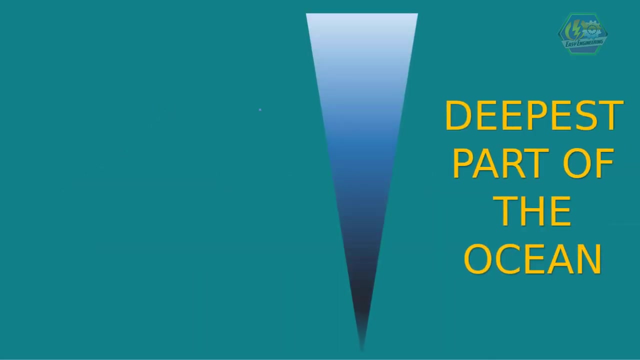 of salty water that covers most of the earth's surface and there are millions of different plants and animals living inside. There are five oceans around the world: The Arctic, Atlantic, Indian, Pacific and Southern Oceans. Fun fact learners: did you know that the Mariana Trench is the deepest part of the ocean? In fact, it is equivalent to how tall the Mount Everest is. Now there are small organisms and bacteria found in the ocean, seas, bays and inlets that make up part of the creatures that live in the marine ecosystem. Where is that possible? There are three main layers of the ocean, based on how deep it is. 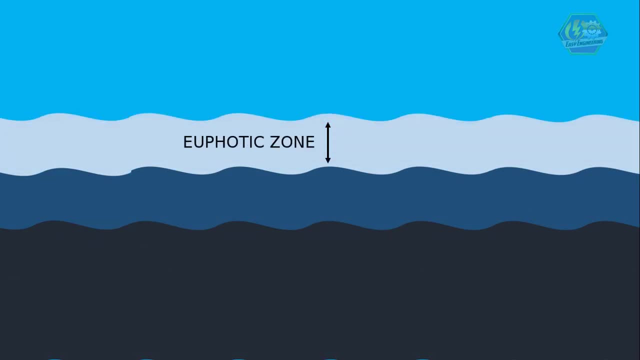 First is the beauphotic, or The Surface Zone. In this zone, sunlight can penetrate or can be seen throughout and the water is warm. Most plants and animals live here. Second is the despotic, or the Twilight Zone. This zone gets some sunlight, but not enough for plants to survive at any moment. 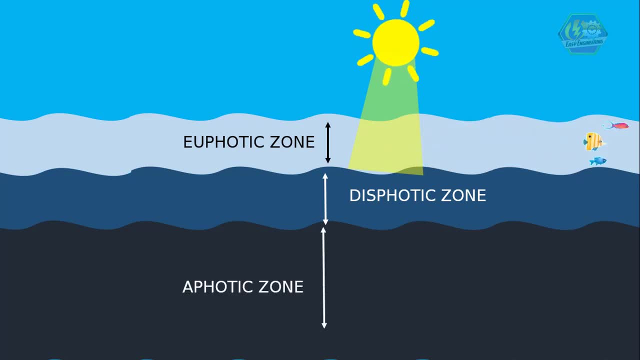 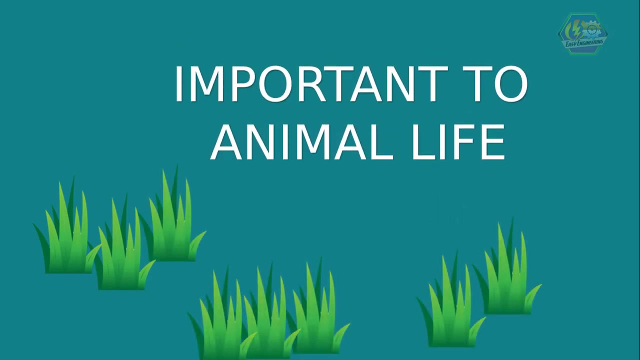 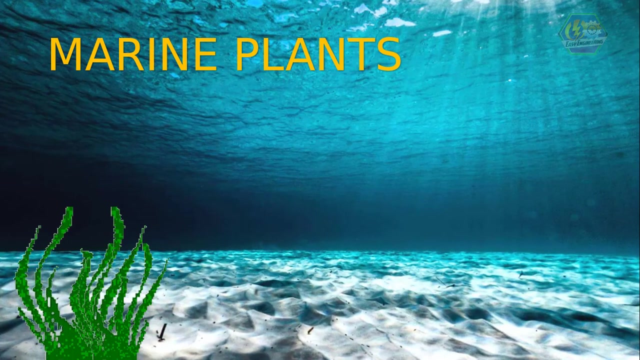 and the third zone is the apoptic zone, where there is no sunlight at all, the darkest side of the ocean where unknown creatures could be lurking. plants serve a very important purpose in the life of animals, but did you know that plants can also grow underwater? some examples of marine plants are the seaweeds marine. 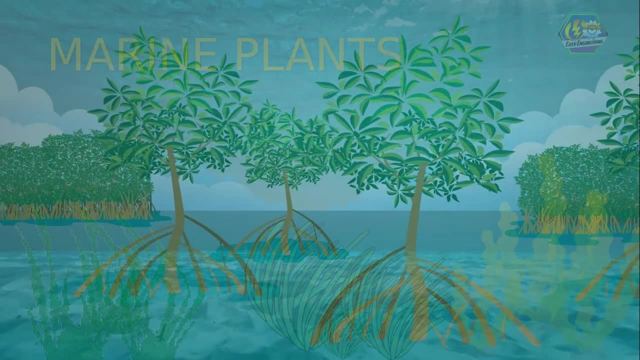 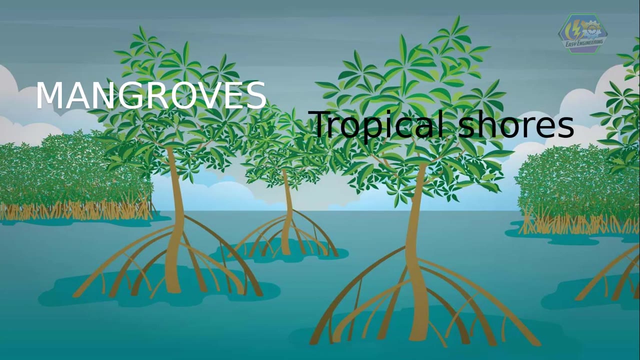 algae and sea grasses. on the other hand, mangrove trees, which live on tropical shores, are also part of the ocean ecosystem. these plants absorb carbon dioxide. in exchange, they give up oxygen for animals to breathe in. marine plants live in the top or euphotic zone of the ocean because they need sunlight to 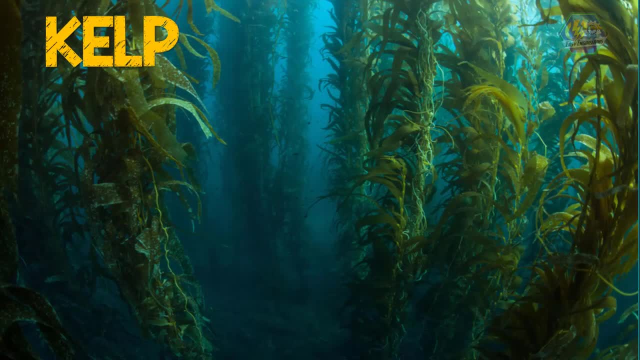 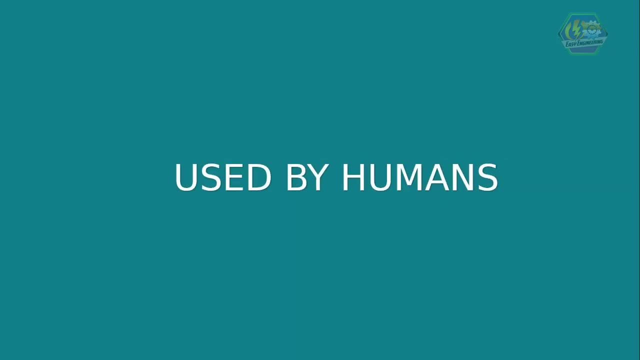 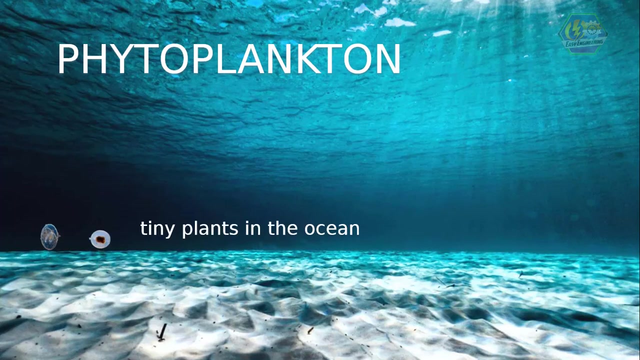 create food through photosynthesis. kelp is a famous type of algae and it provides food and shelter to ocean animals. did you know that it is even used by humans in things like ice cream and toothpaste? phytoplankton are tiny plants in the ocean that serve as the 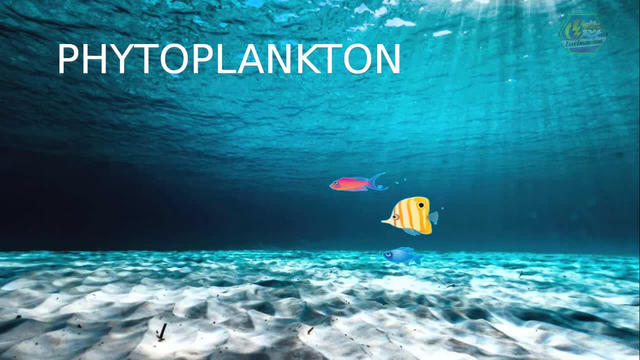 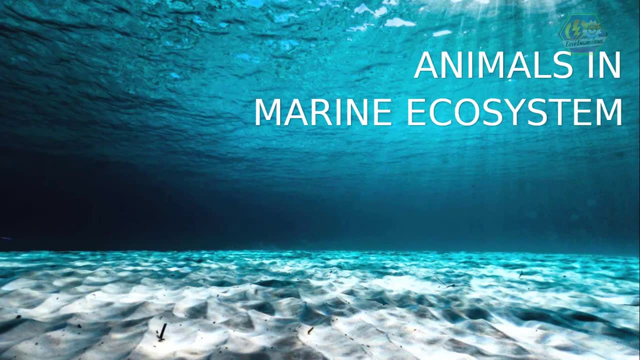 food for many ocean creatures, like smallest fish and even the largest of whales. speaking of animals, what animals found in the marine ecosystem? I'm sure there are lots and lots of them that we couldn't even count, since the ocean is vastly wide, the ocean is a very large ocean and the ocean is a very large. 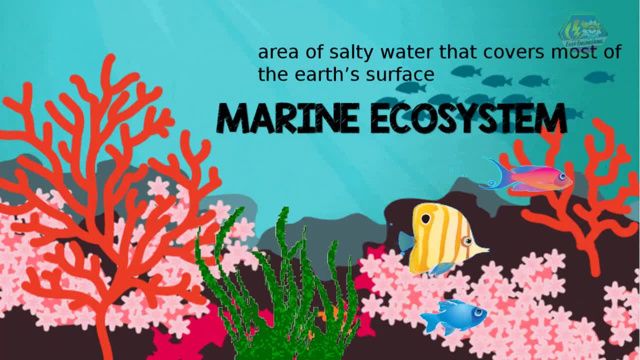 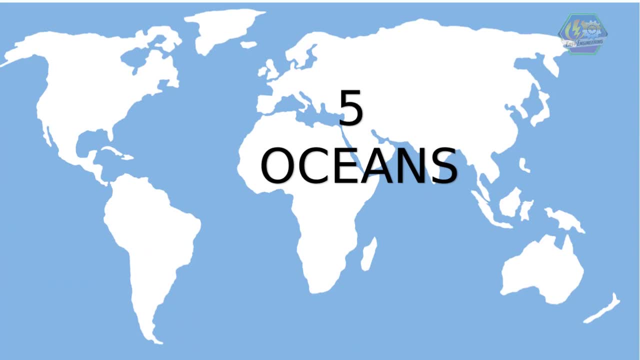 of salty water that covers most of the earth's surface, and there are millions of different plants and animals living inside. The marine ecosystem is made up of three main parts of the ocean: the Arctic, Atlantic, Indian, Pacific and Southern Oceans. 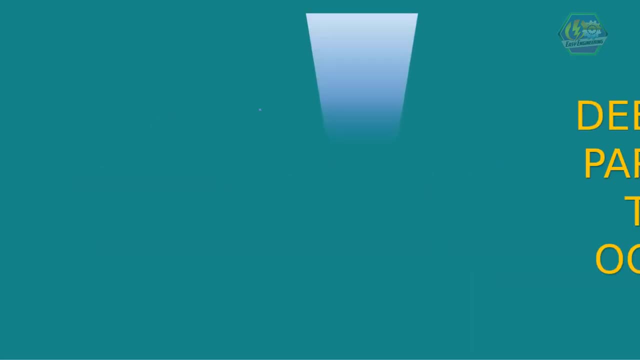 Fun fact learners. did you know that the Mariana Trench is the deepest part of the ocean? In fact, it is equivalent to how tall the Mount Everest is. Now there are small organisms and bacteria found in the ocean, seas, bays and inlets. 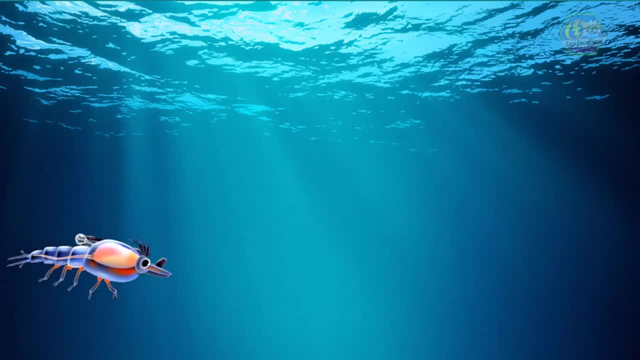 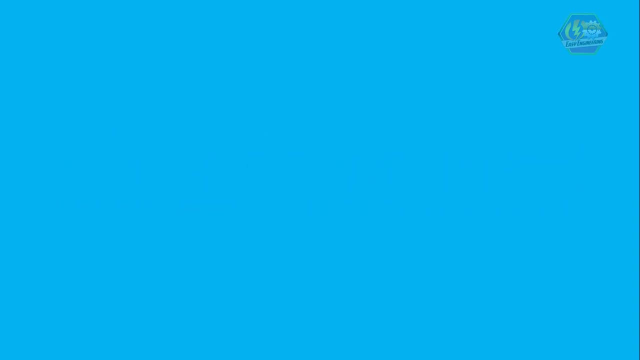 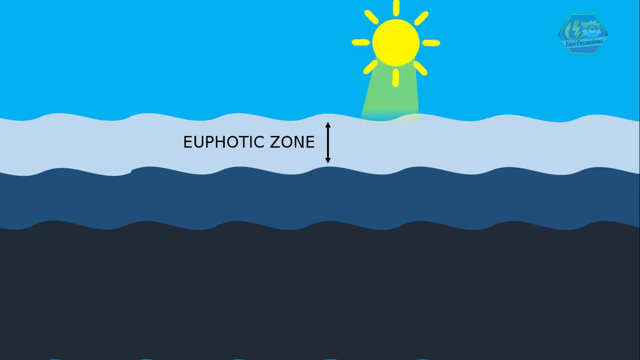 that make up part of the creatures that live in the marine ecosystem. There are three main layers of the ocean, based on how deep it is. First is the euphotic, or the surface zone. In this zone, sunlight can penetrate or can be seen throughout and the water is warm. Most plants and animals live here. 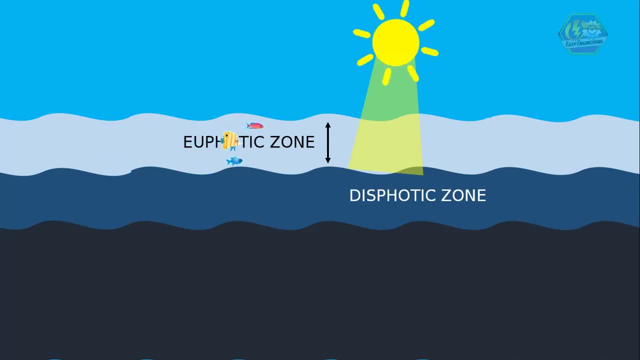 Second is the despotic or the twilight zone. This zone gets some sunlight, but not enough for plants to survive. And the third zone is the apothic zone, where there is no sunlight at all, The darkest side of the ocean where unknown creatures could be lurking. 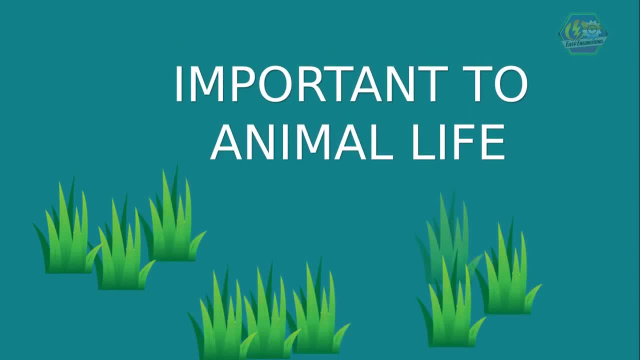 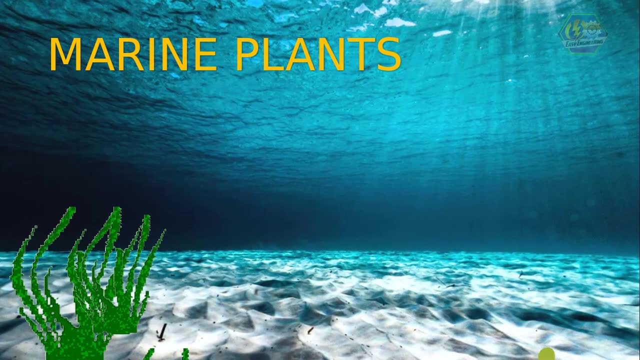 Plants serve a very important purpose in the life of animals, but did you know that plants can also grow underwater? Some examples of marine plants are the seaweeds, marine algae and sea grasses. On the other hand, mangrove trees, 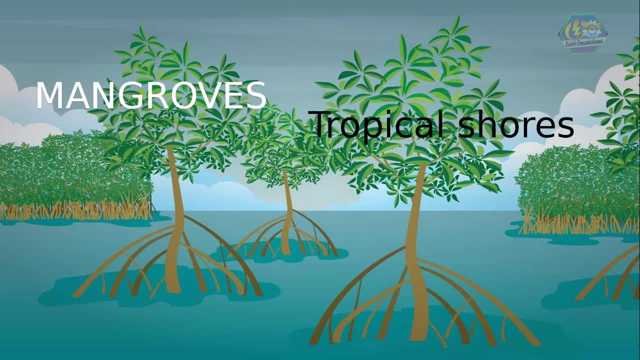 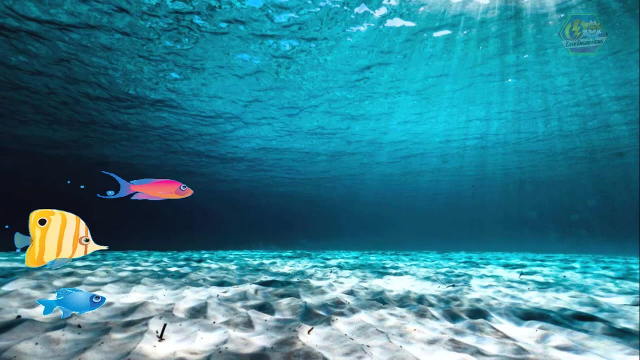 The mangrove trees, which live on tropical shores, are also part of the ocean ecosystem. These plants absorb carbon dioxide. In exchange, they give off oxygen for animals to breathe in. Marine plants live in the top or euphotic zone of the ocean because they need sunlight. 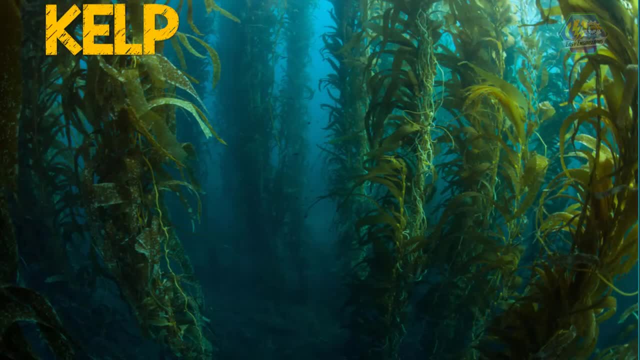 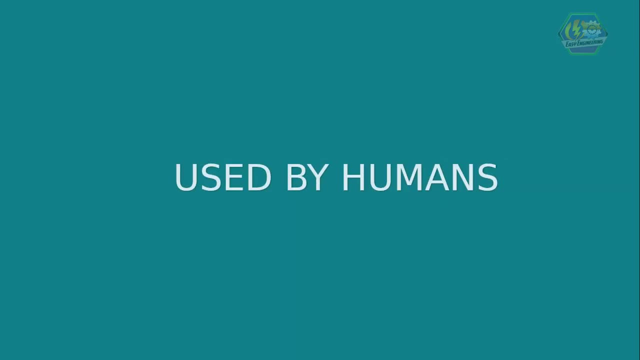 to create food through photosynthesis. Kelp is a famous type of algae and it provides food and shelter to ocean animals. Did you know that it is even used by humans in things like farming? The kelp plant is also known as the mangrove plant. The mangrove plant is also known as. the mangrove plant. The mangrove plant is also known as the mangrove plant. The mangrove plant is often used for soil, Anaesthetics, water saving and genitalia. If you want to know how beautiful mangrove plants exist, why would you buy it? 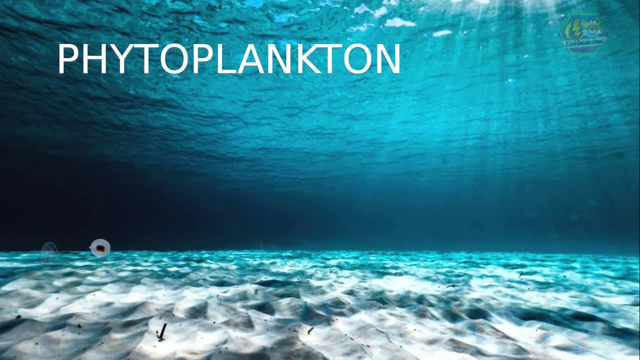 D Ages back to 1780s. Planets impressiveías Like ice cream and toothpaste. Phytoplankton are tiny plants in the ocean that serve as the food for many ocean creatures, like smallest fish and even the largest of whales. Speaking of animals, what do we find in the marine ecosystem? 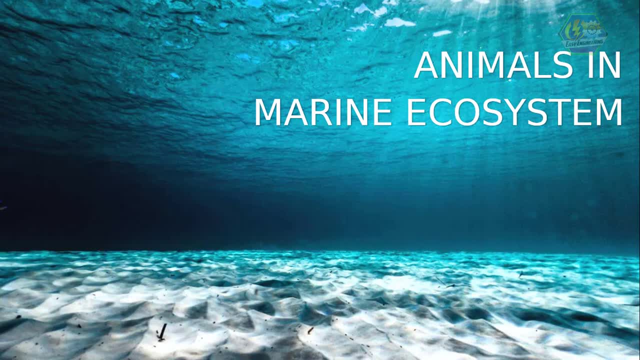 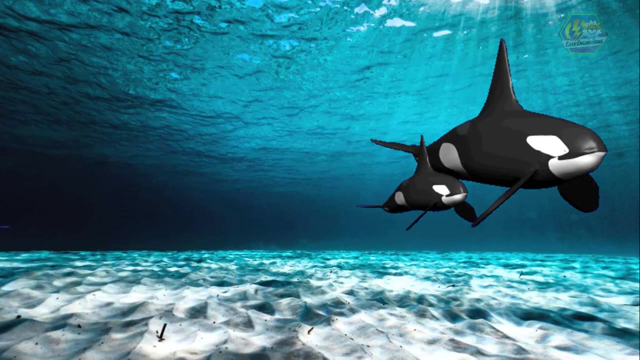 I'm sure there are lots and lots of them that we couldn't even count, since the ocean is vastly wide. The ocean consists of a large variety of animal life, including fish, mollusks, dolphins, seals, walruses, whales, crustaceans, bacteria, sea animals and many. 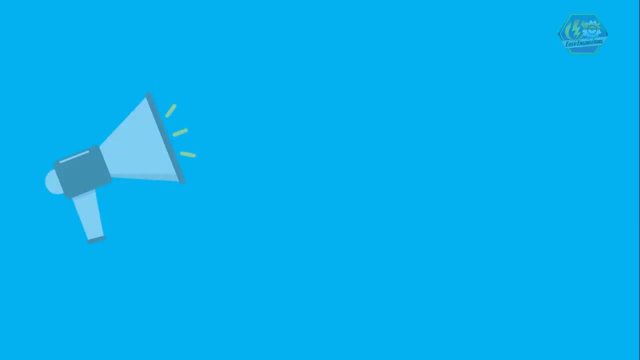 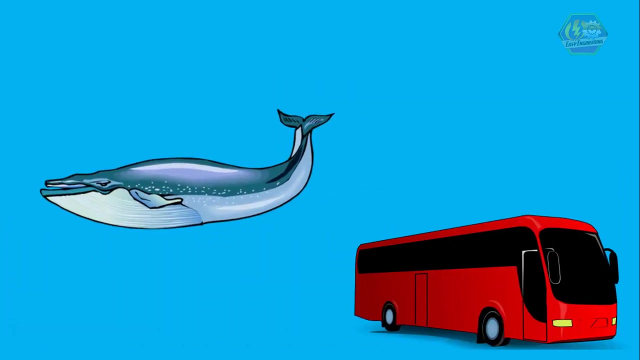 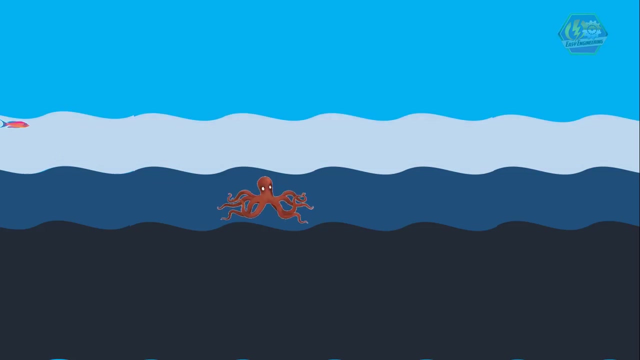 others. fun fact learners. did you know that the largest animal in the sea is the blue whale? it averages up to seven point six meters long at birth and weighs about three tons as an adult. it can easily stretch to the length of a city bus and weigh close to 200 tons. now back to the topic. most marine animals stay in. 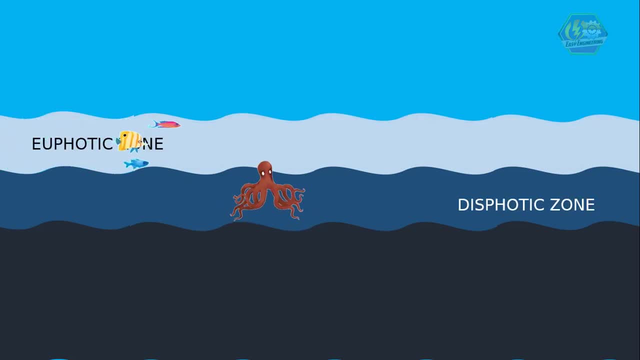 euphotic and dysphotic zones where they have access to plants and other ocean animals to eat. but deep down below the layers there is life too, and they might look weirdest animals on earth. one example is the angler fish. fishes like this adapt to the darkest side of the ocean. 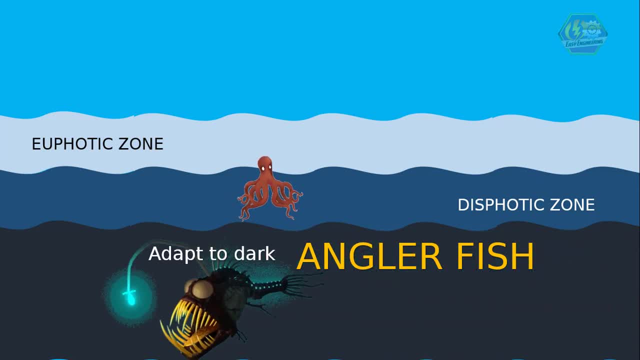 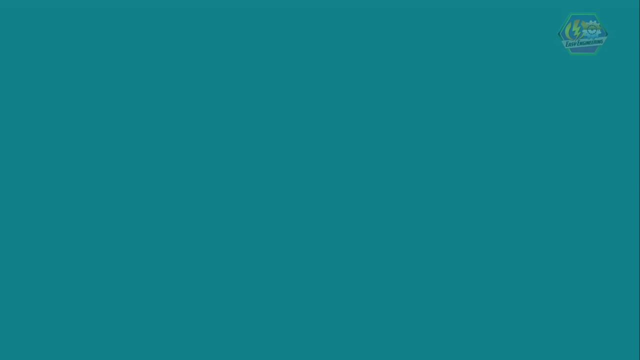 you can find them anywhere in the world. in fact, the angler fish creates its own light to lure their prey, and when it is close, the angler fish just gobbles it up in a blink of an eye. we humans use the ocean a lot, whether it's for food, medicines, oil, other resources or just for 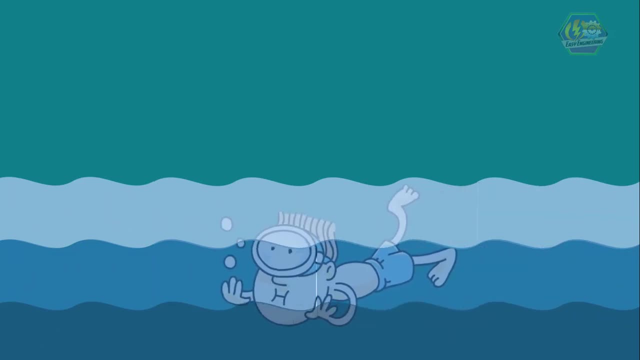 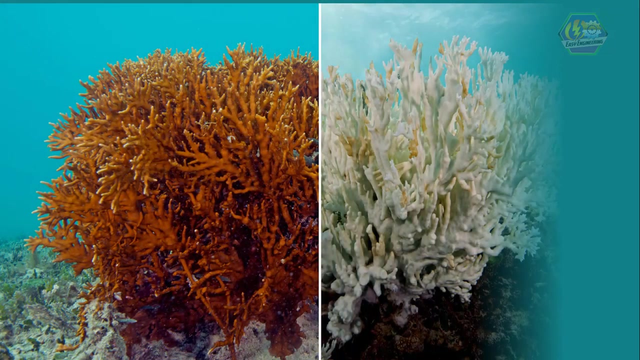 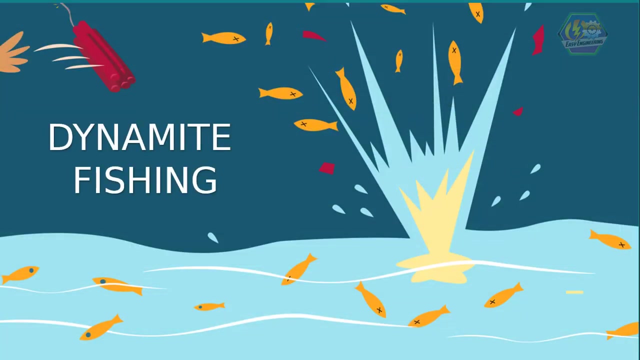 recreation like swimming and parties. either way, we love the things that the ocean gives us, but the demand for resources from the ocean can be destructed to their marine ecosystems around the world. bad fishing practices, like poisoning and using dynamites to catfish, also kills other. 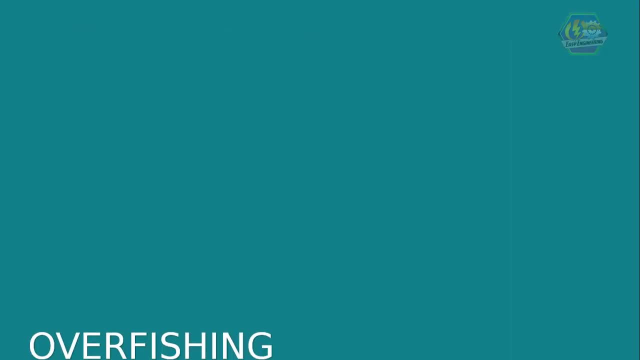 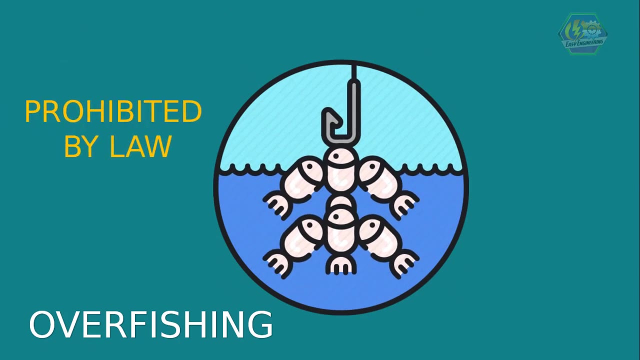 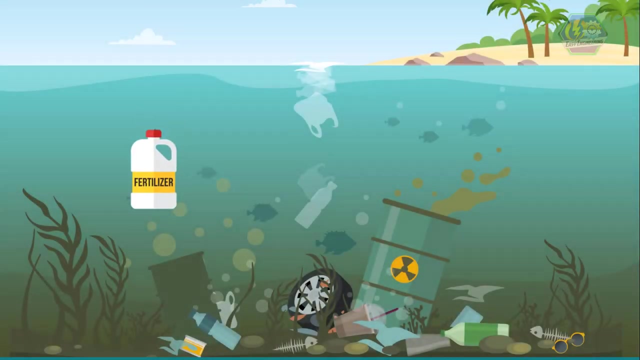 animals like corals and small fishes. over fishing popular species and endangered species are prohibited by law, but some people still do. pollution is és också harming the marine ecosystem. pollutant such as fertilizers and household products. E entendong quereko pangas. 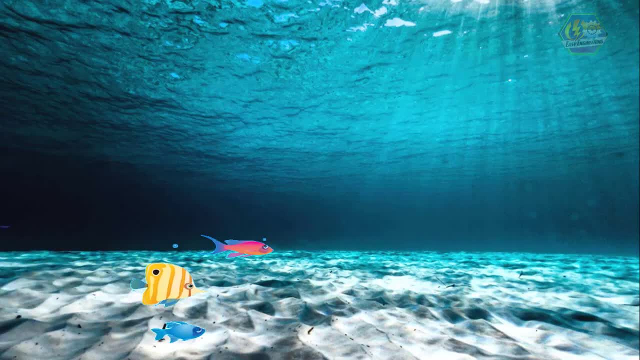 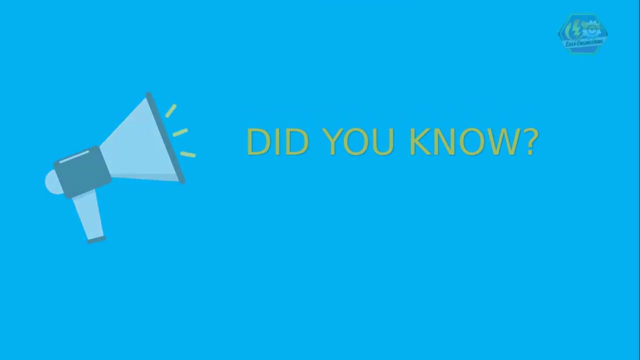 ocean consists of a large variety of animal life, including fish, mollusks, dolphins, seals, walruses, whales, crustaceans, bacteria, sea animals and many others. fun fact learners: did you know that the largest animal in the sea is the blue whale? it averages up to seven point six meters long at birth and weighs. 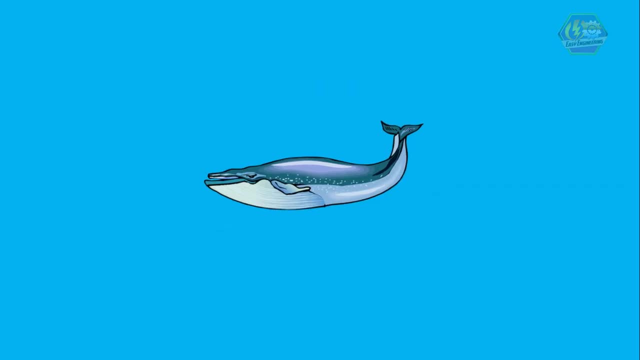 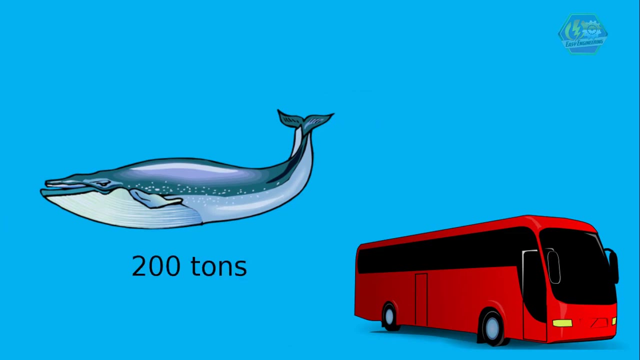 about three tons. as an adult it can easily stretch to the length of a city bus or arctic bus to the sea. it can be a couple of days long and after some, and weigh close to 200 tons. now back to the topic. most marine animals stay in euphotic. 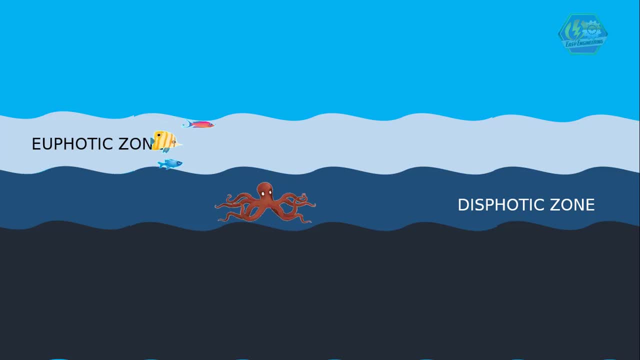 and dysphotic zones where they have access to plants and other ocean animals to eat. but deep down below the layers there is life too, and they might look weirdest animals on earth. one example is the angler fish. fishes like this adapt to the darkest side of the ocean. 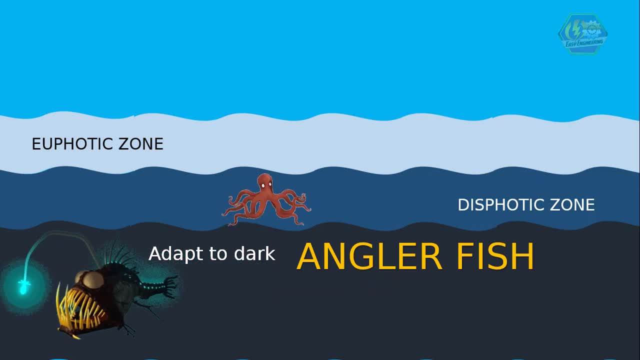 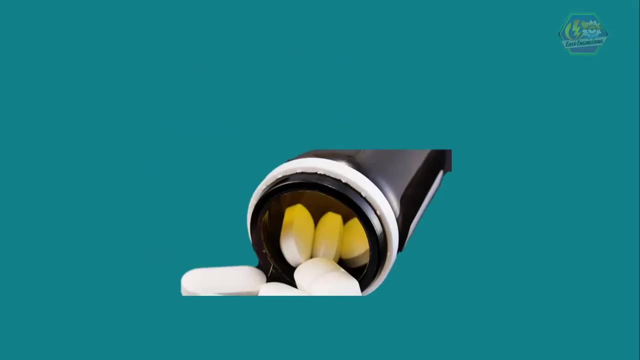 in fact, the angler fish creates its own light to lure their prey, and when it is close, the angler fish just gobbles it up in a blink of an eye. we humans use the ocean a lot, whether it's for food, medicines, oil, other resources or just for recreation like swimming and 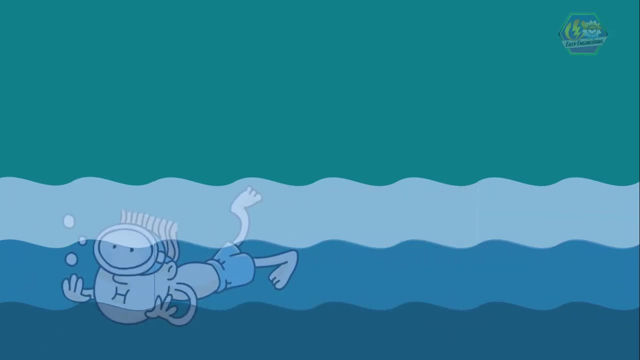 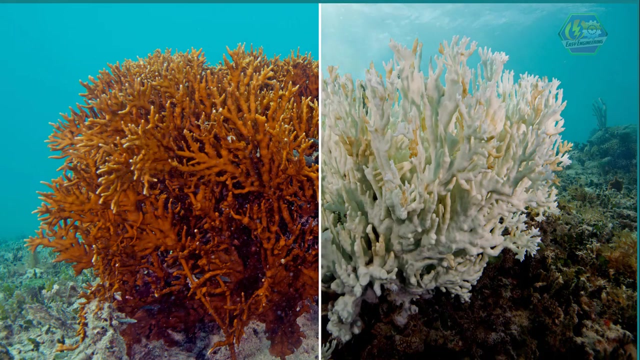 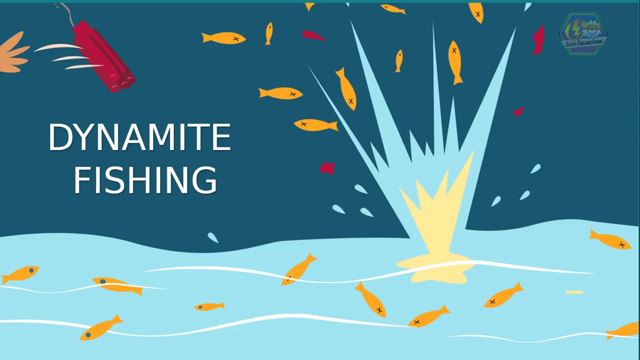 parties. either way, we love the things that the ocean gives us, but the demand for resources from the ocean can be destructive to the marine ecosystems around the world. bad fishing practices, like poisoning and using dynamites to catfish, also kills other animals like corals and small fishes. 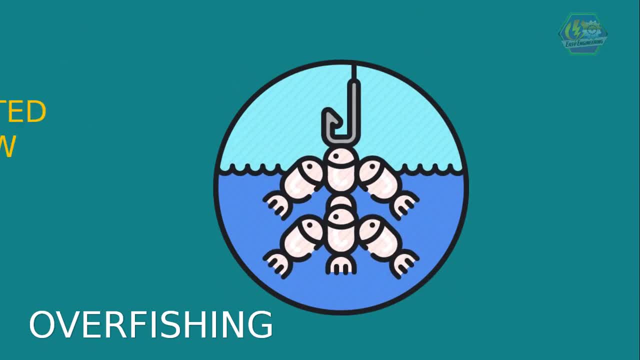 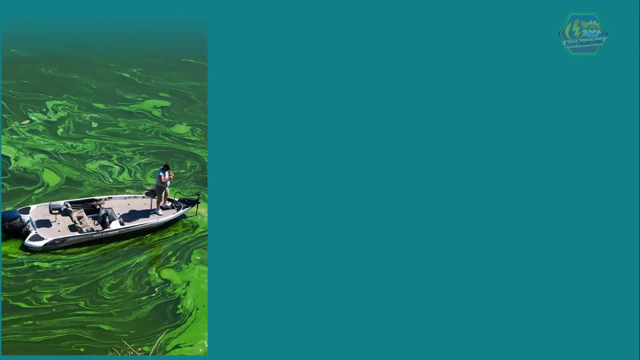 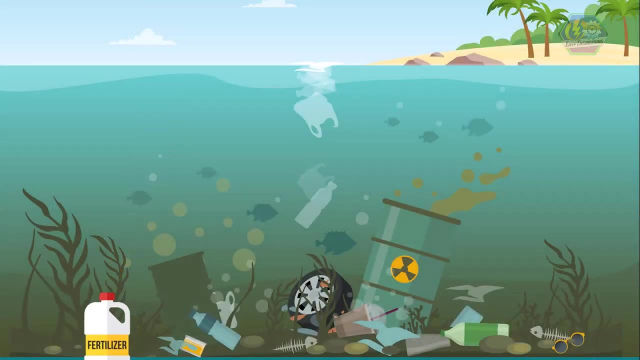 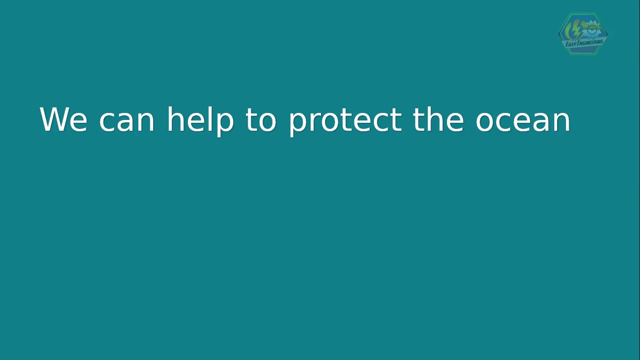 over fishing. popular species and endangered species are prohibited by law, but some people still do it. pollution is also harming the marine ecosystem. pollutants such as fertilizers and household products, and even oil spills ruin the beauty of the ocean for us. there are many simple things that you can do to help protect the ocean.